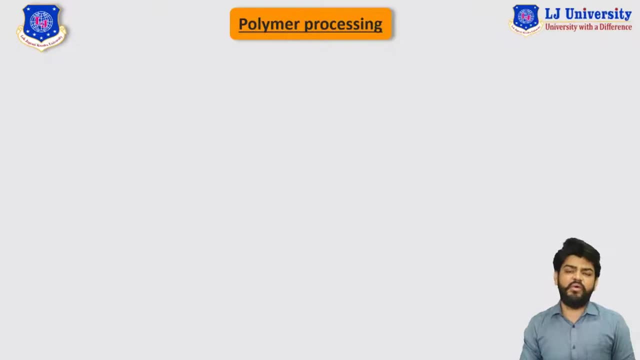 of polymer processing and we have introduced various terms in this chapter and we have started the discussion on the compression molding. If you have missed that video, you can find it in the i button on the top of this video. So now, having said that, let us just further continue our discussion on the compression. 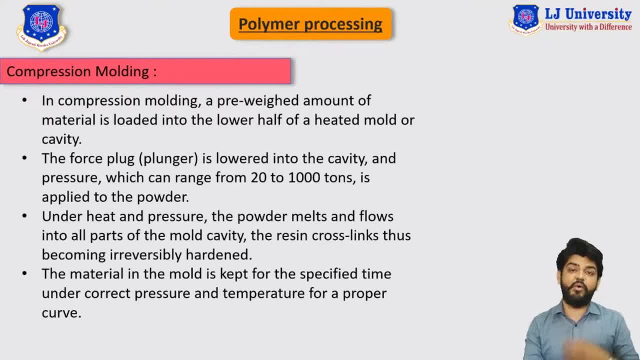 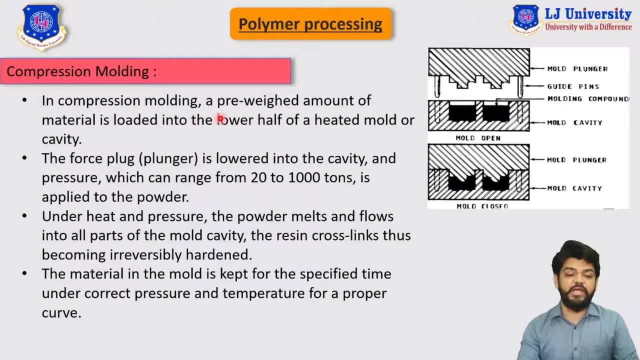 molding. Let us just quickly revise what we have understood in the compression molding in a previous lecture. So we have seen that in a compression molding a pre-weighted amount of material is being loaded into the lower half of the mold. So we have seen that in a compression molding a pre-weighted amount of material is being loaded into the lower half of the mold. 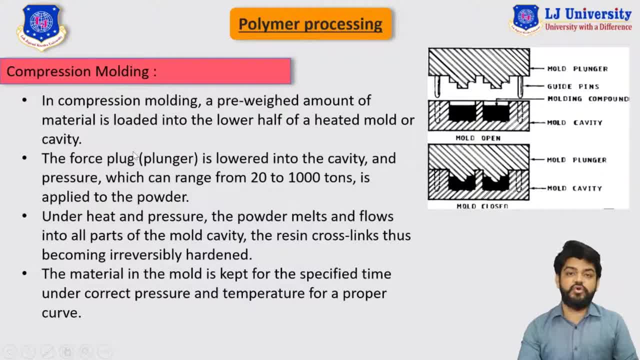 So we have seen that in a compression molding, a pre-weighted amount of material is being loaded into the lower half of the mold or the cavity. So, as you can see here in this image, a pre-weighed raw polymer that is melted and is being 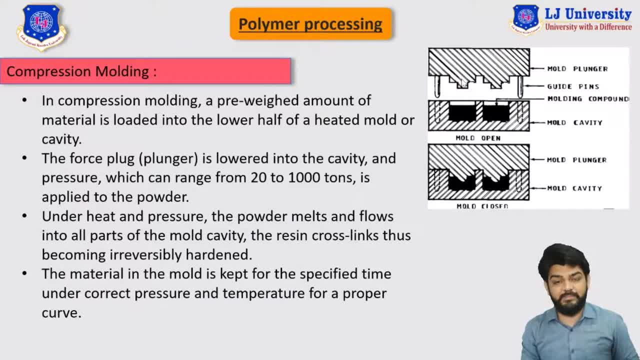 injected inside the cavity, right? So, as you can see here, this is our mold and we find that it is inside the cavity. So initially the pre-weighted polymer is being inserted or filled inside the cavity of the mold. Now, later, the force, or we can say plug, is lowered into the cavity and pressure which 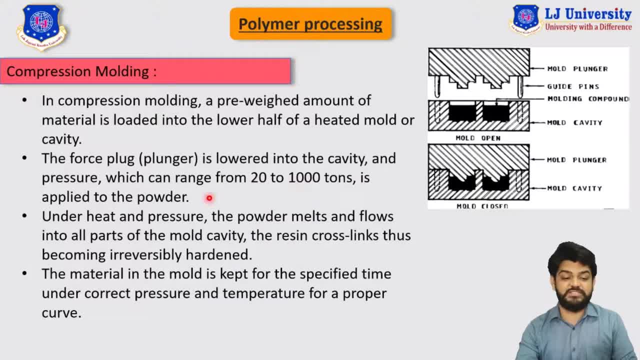 can range from 20 to 1000 tons, is applied to the powder. So, as you can see here on the screen that now this is the plunger or the plug that we are discussing, The weight or the pressure applied by this plug may vary from 10 to 1000 of the ton, right? 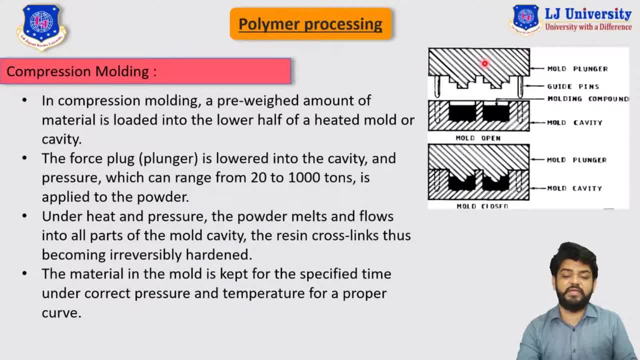 So when this plug or the plunger is being forcefully pressurized on this molten form of the polymer, right? So this is the process of the compression molding. Now let's see what is the next step in this process: Under the effect of heat and pressure, the powder or the raw polymer that we have converted 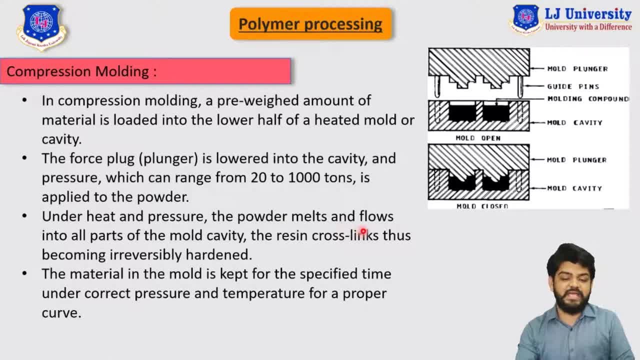 into the molten form. the powder melts and flow into the all part of the molten cavity. The resin crosslinked thus become irreversibly hardened. So as a effect of the heat and temperature, this molten form of the polymer or the polymer powder, whichever form of polymer you have taken, is now been converted and it will be. 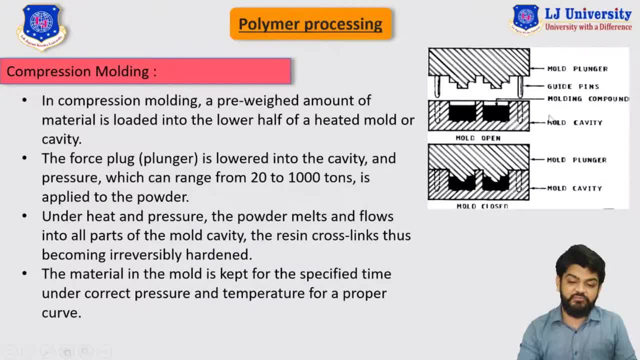 filled all the parts of the cavity right. It will fill all the part of the cavity and it will generate our useful desired polymer material Right. Then the last step is that the material in the mold is kept for specified time under correct pressure and temperature for the proper curve. 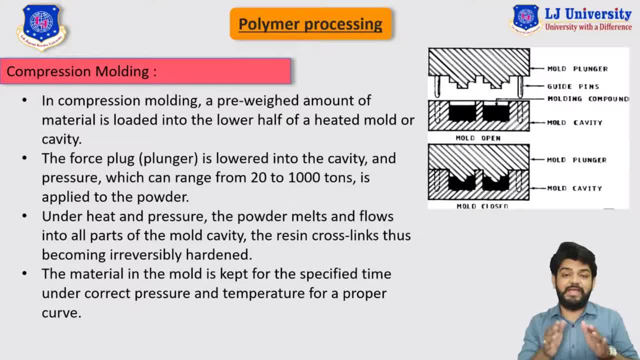 So as a result now, our polymer will be kept inside the mold for specific amount of time under the pressure and temperature effect, so that all the curves of our desired shape or the mold will be taken by the polymer itself. So, as you can see here, 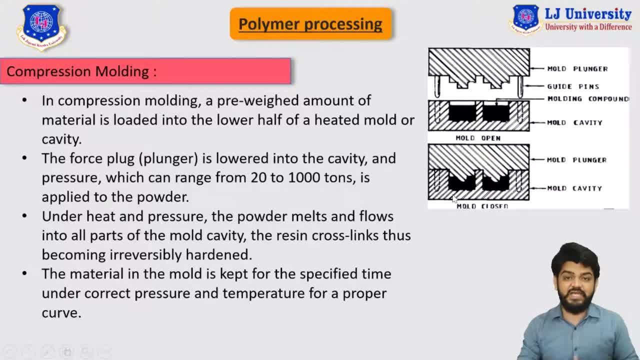 Now we have closed our mold and we are resting it for a some specific amount of time so that it can easily adapt the shape of the polymer right, or you can say the shape of the mold, So that the shape of the mold can be achieved by the polymer. 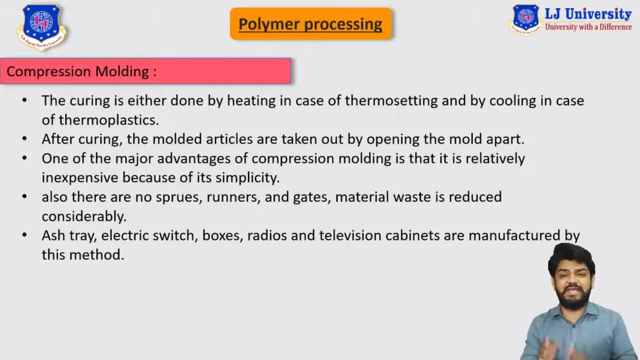 Now, if we discuss further more about this, then the next steps come. is that the curing? So, as you can see here, the curing is either being done by heating, In the case of thermosetting polymers, and by cooling, in the case of the thermoplastic. 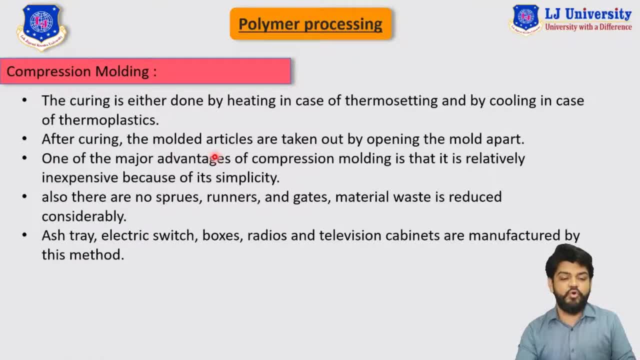 polymers, after curing the molded article, are being taken out by opening the mold apart. So now what we are going to do is we will open our mold and the molded article, that is, our polymer, or desired shape of the polymer, is being taken out from the mold. 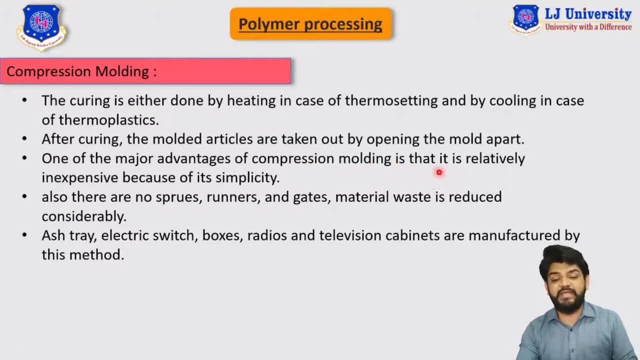 One of the major advantage of the compression molding is that it is relatively insoluble. It is relatively inexpensive because of its simplicity. So, as you have seen in the previous image, that this polymerization technique is very simple and hence it is the most inexpensive method for the production of the molten polymers. 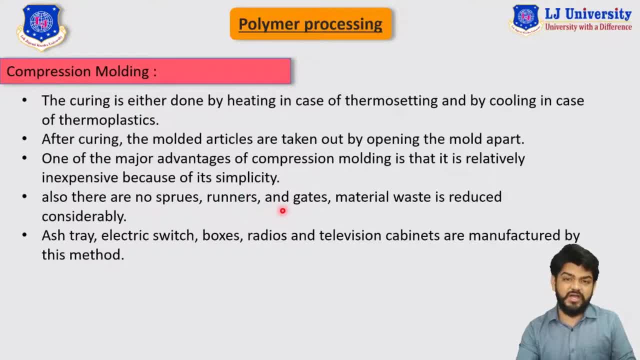 right. So there are no spurs, runners and gate, then material waste could be wasted. So there are chances of waste of raw material is very minimum with the compression molding. As there are no spurs, runners and gate, then material waste could be wasted. 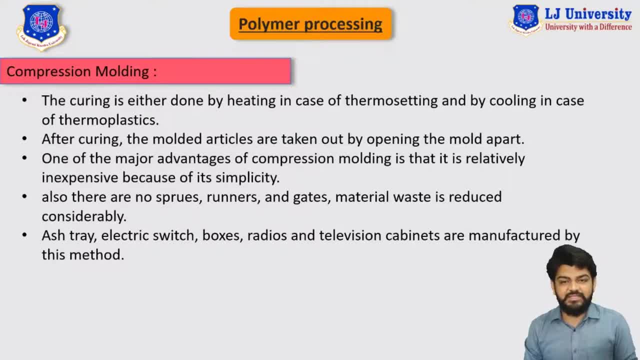 As there are no spurs, runners and gate, then material waste could be wasted. As there are no much of the complicated parts, there is only one mold which is responsible for the getting the desired shape of our polymer As tray, electric switch box, then radio television cabinets, all are the different. 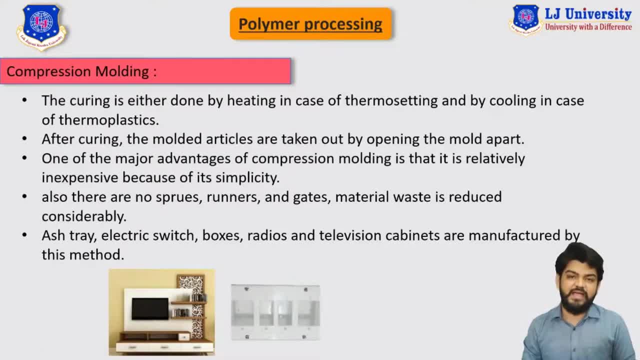 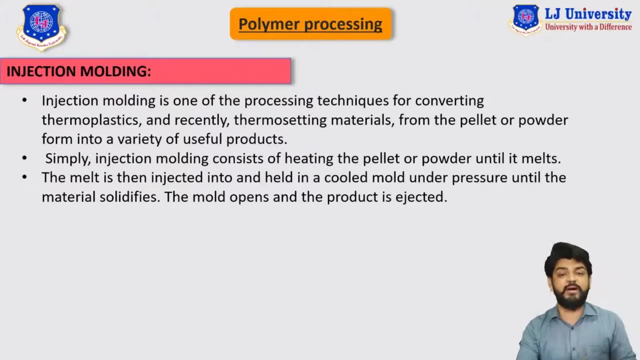 examples of this compression molding. As you can see here, this switch module is easily be constructed with the help of compression molding. As you can see here, this switch module is easily be constructed with the help of compression. this was all about the compression molding. Now let's just further discuss about the injection. 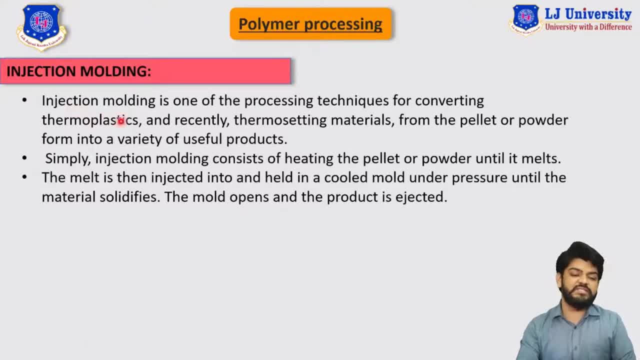 molding techniques. So, as you can see here, injection molding is one of the processing technique for converting thermoplastic polymers And recently there have been technologies which are being developed to convert even thermosetting materials by means of the injection molding From the pellets or the powder form of the different varieties of the raw material. 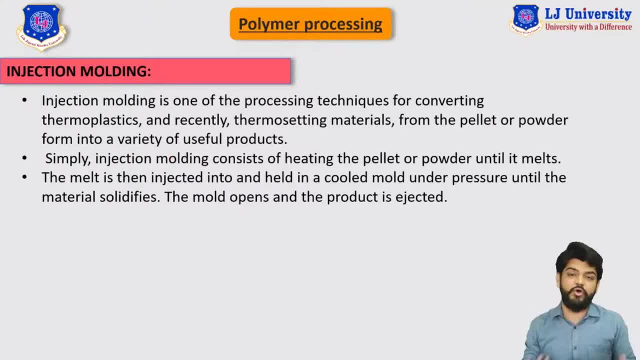 we can convert it into the desired shape of the polymer by means of the injection molding techniques. This injection molding techniques are again very important for the exam, point out, as it is being largely used in an industrial application as well. So let's just understand what are the different steps and how this injection molding polymerization techniques. 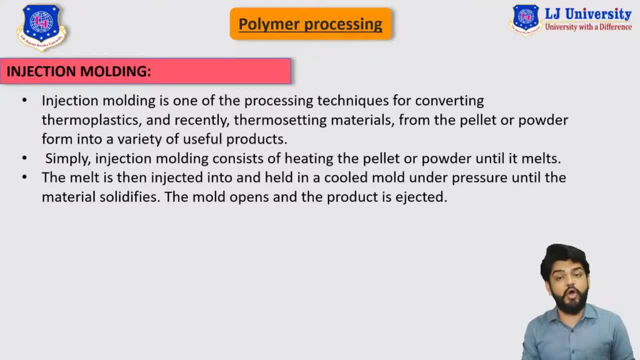 is being performed to get desired shape of our polymer. So, as you can see here, our injection molding simply consists of heating the pellets or the powder until they melts down. so as the first step, we are targeting our powdered form or the molten form of the polymer to get melted down. so the first step in the injection molding 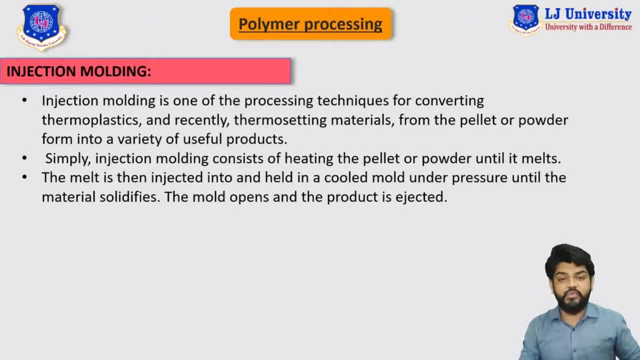 is to prepare a molten form of our powder or the pellet form of the polymer. right then. the melt is then injected into the. then this molten form of polymer is then injected and held in the cooled, molded under the pressure, until the material is get solidified. so now, 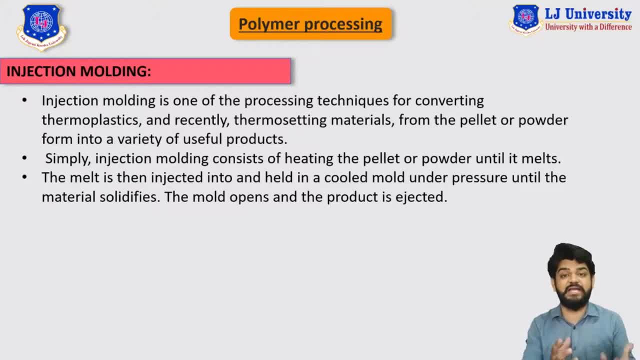 this molten form of the polymer is being injected inside the injection molding unit. and on the effect of cooling, we are applying some and we are applying effect of cooling until our polymer ultimately gets solidified. Then the mold is being opened and our product is being taken out. right, there are, if we discuss, 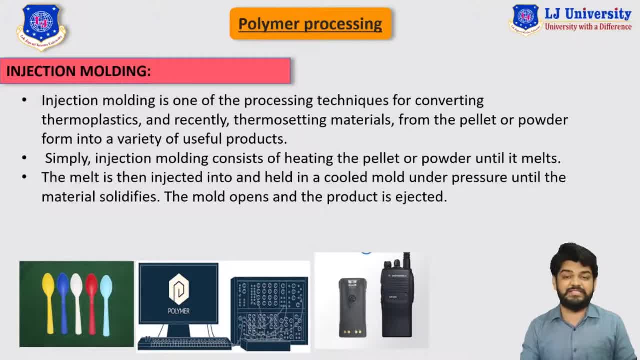 about the examples of the injection molding techniques, then different types of this spoon frogs, then our computers, then the different radios are being manufactured by this injection molding type of the technique. there are different parts and compartment in the injection molding unit. Let us see what are the functions of this injection molding. 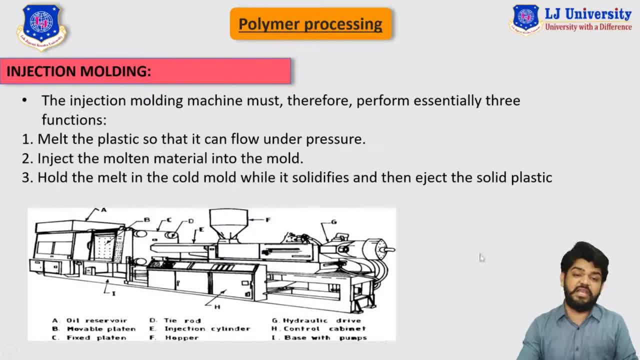 injection molding right as you can see here on the screen that the injection molding machine must therefore perform essentially three functions. so, basically, there are three main functions that need to be followed by the injection molding, and those functions are: melt the plastic so that it can flow under the pressure. so the first function of this injection molding machine is to melt down our 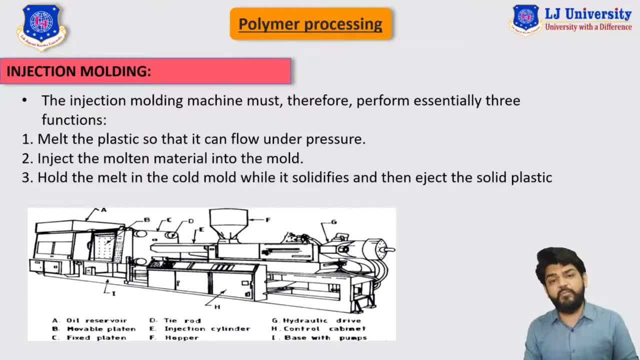 plastic raw polymer right, so that this molten form of the polymer can be easily flow from one part to another part. then the second function is that inject the molding material into the mold. so the second function that need to be performed by the injection molding machine is that to insert our 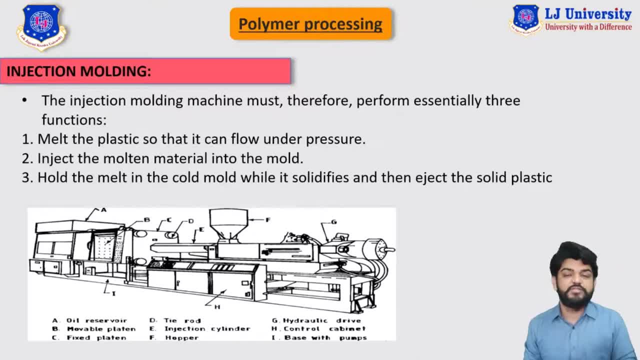 molten form of the polymer inside the mold so that it ultimately gets its desired shape. and the last function is that hold the melt in the molding machine so that it can flow under the pressure in the cold mold while it solidified, and then eject the solid plastic. so there should be some specific 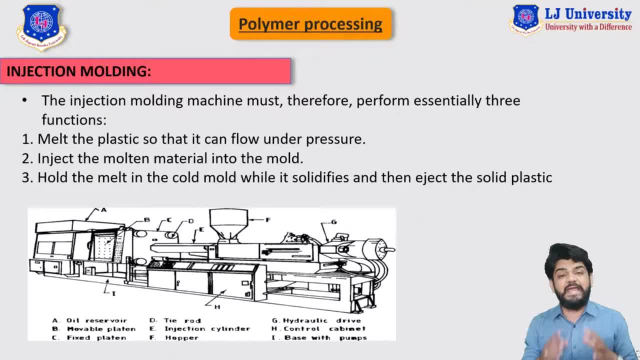 amount of the time which is need to be predefined for that particular time. our injection molding machine should hold our molten form of the polymer inside the cold environment of the mold right and ultimately, as a result, we get the desired shape of the polymer and then shape should be ejected from. 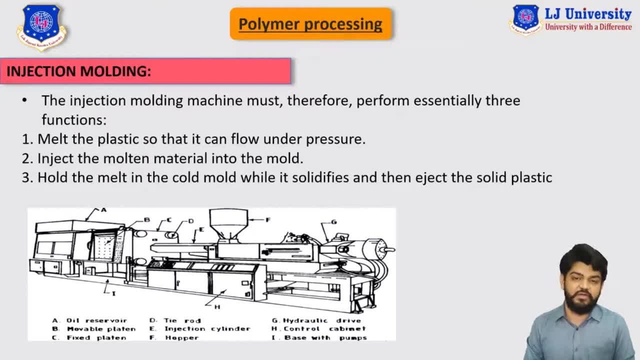 the bolt of the injection molding machine. so, as a result, you can see here the typical image or the typical schematic diagram of the injection molding machine. it contains different shapes right from this particular type. a whopper is there, which is represented by f, inside which we are inserting our 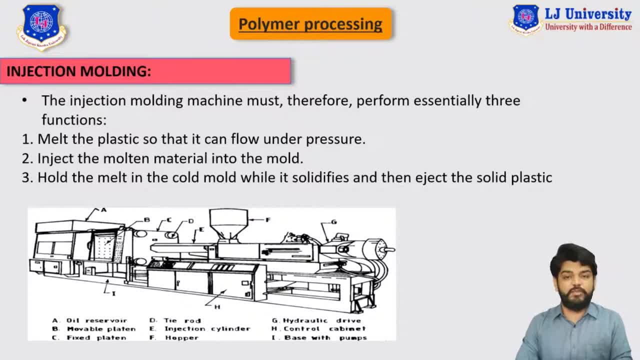 powdered form of the polymer or the or the pellet form of the polymer. that polymer can be converted into the molten form on the application of the heat and the molten form of the polymer. and then we can see it here in our new mould, in our mold paste. we are inserting our plasticized screw into the mold. 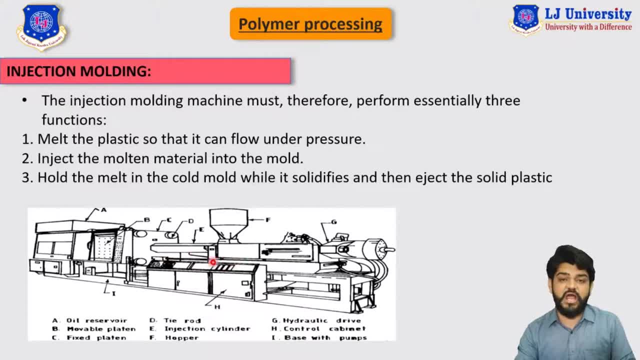 and this ända on the compassion with, and the second one is the plasticized screw which is inside this unit right, which actually transport our molten form of the polymer inside the moves right. so it is the major and main component which actually transfer her molting. form of your polymer inside the mold, so that, or polymer, we'll get the desired shape of the mode. now let's just further discuss without the next technique of the mold, and then we are done. this machine keep massating for the next stage of the air. tough, originally emptyréponementOffice- whiting playful avoir. 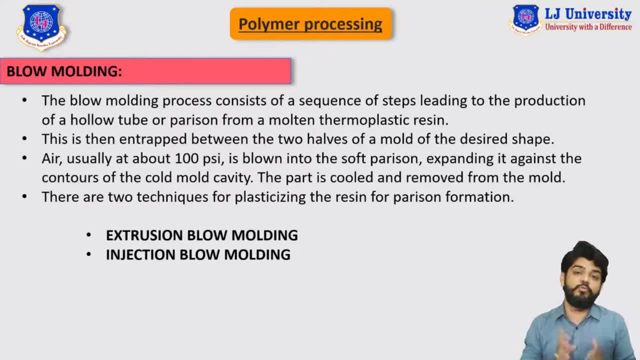 polymerization process and that is blow mold. So, as you can see here on the screen that the blow molding process consists of a sequence of the step leading to the production of a hollow tube or prison from the mold and thermoplastic resin. So this particular type of the method is being used to 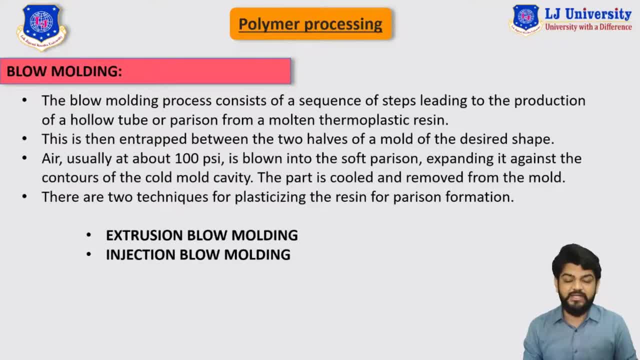 produce hollow type of the polymer product, such as plastics or different types of the tube, even a ball or such kind of a thing, which are essentially of the shape of hollow, which are essentially hollow in a shape. This is then interrupt between two halves of the mold, of the desire shape. So such kind of the 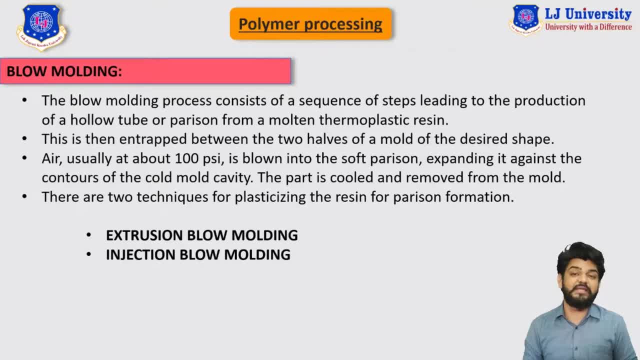 polymer, that are our thermoplastic polymer, is being injected into the mold by the two halves of the molding machine, And then air- is usually about my 100 psi- is being blown into the soft prison and expanding it against the counters of the cold mould cavity. 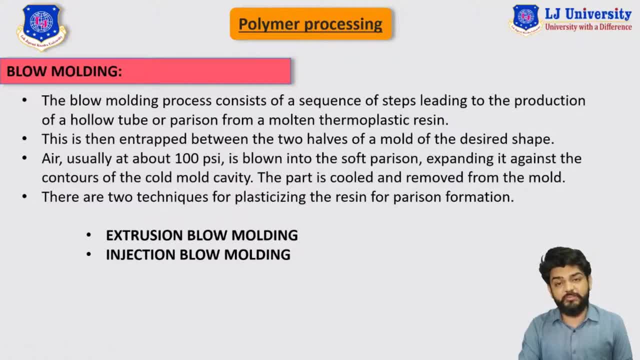 So now we have injected our molten form of the polymer inside the cavity. after that we pass air of the pressure around 100 psi so that our polymer, or the molten form of the polymer, will get desired shape of the mould. and this is how we can actually produce the